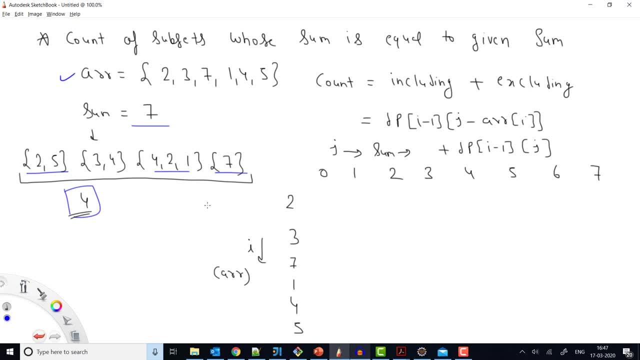 basically take care from the starting and we'll just consider the basic cases and, using the solution of the basic cases, then we'll find out the up solutions. so, like what it means, it means of all, we'll check that, let's say, if we have only one set, if we have only one value in two, 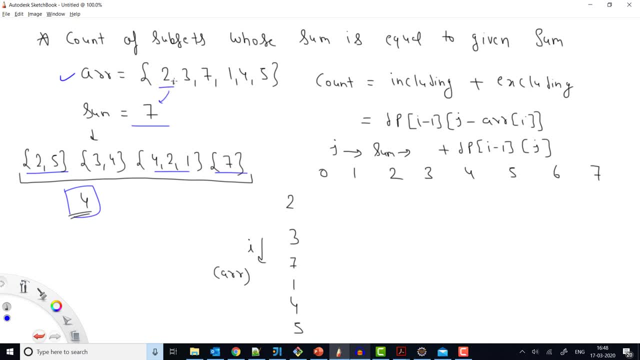 then how many subsets are there which is making seven? so once we found out with two, then we'll check with the two values. then it will check that, let's say if it is a, if it has only two values in subset. so how many subsets are there which is making some right? then we'll check with the three. 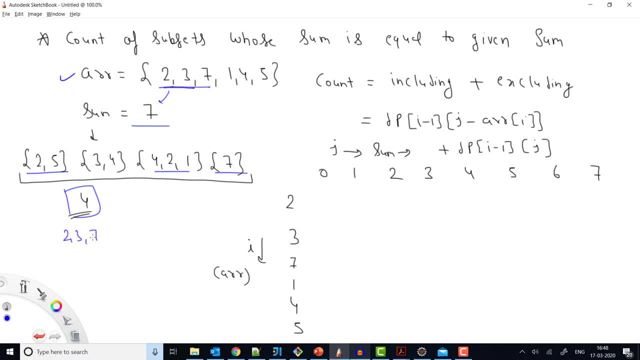 subset. so three subset means we'll check that. if let's assume that we have only three values in my set, that how many values are there, which is making some 7? then we will check with the 4 values- 2, 3, 7, 1- then we will check with the 5 values, then we will check with the. 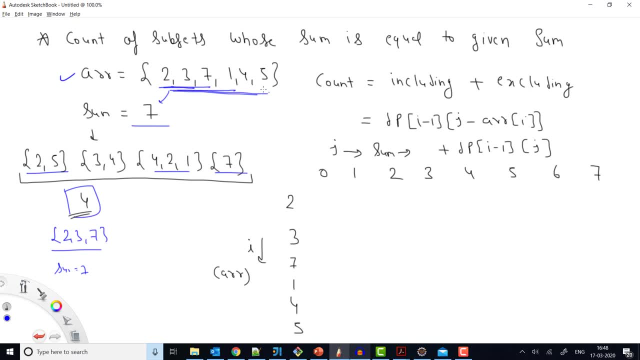 6 value and whatever will be the 6 value at the last, then we will return our answer right. so the point is that how I will represent this structure right? so basically we represent it as 2D array. so basically we will solve it as 2D array and we will define sum: the sum we will define as a sum. 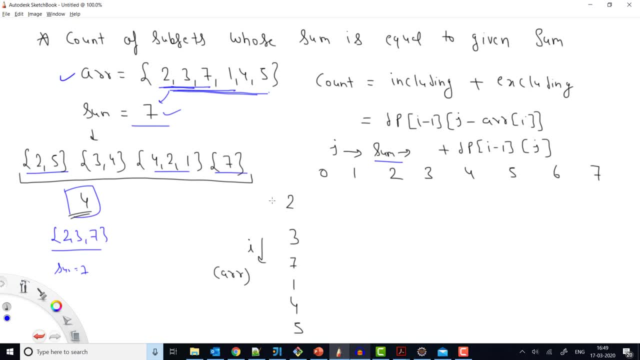 in the column manner and we will define and we will define all the array element in the row manner. right? so here, when I am defining this one, when I will calculate on this row, it means I am calculating only on the one set, lets say, if it has only one element. 2. 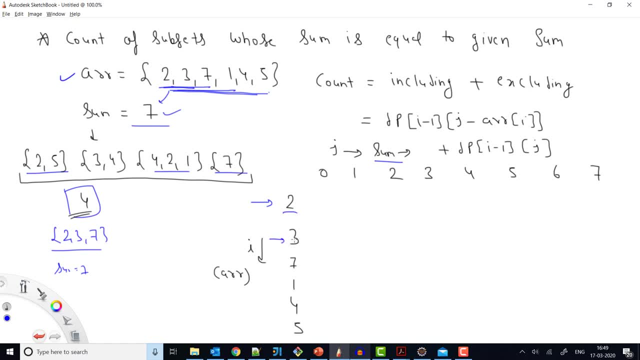 now when I will appear in this row, it means my current element is 3, but my mean is that basically I have 2 element as of now when I will operate on this one. basically it means that I have 3 elements here, right when i'm operating this one. then i have four element when i'm operating this one, when 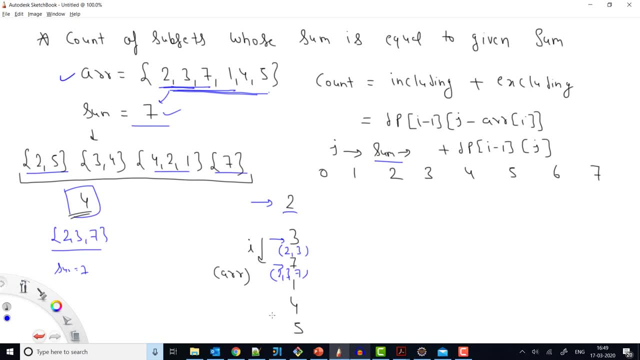 then i have five element and when i will operate on this one, then i will have all the six element right. similarly, on the column side i represent something like this: that this is the sum when you have. when you have sum equals to zero, it means how many subsets are there, whose sum is. 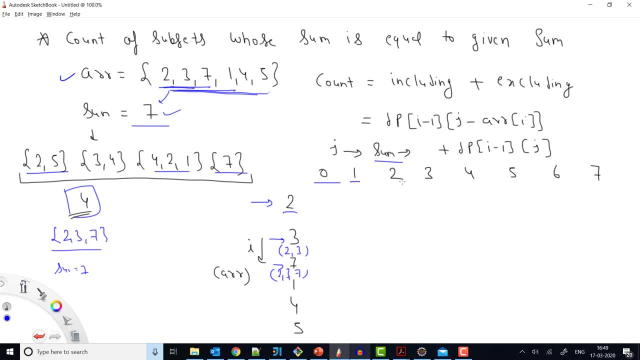 equals to zero, or how many subsets are there whose sum is equal to one, two, three, four, five, six, seven, right? so basically, if you observe here what we are doing, we are always calculating from the bottom solution. let's calculate the, the count of the subset when your sum is zero. count of the subsets. 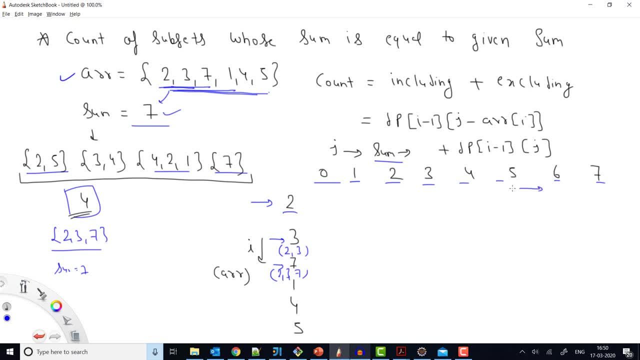 when your sum is one and then we are going further, right? so when we will fill the values, then you will see, basically, using the solutions of the sub problem, then we'll find down, then we'll find out the further solutions and similarly, here we are saying that let's check when you have only one. 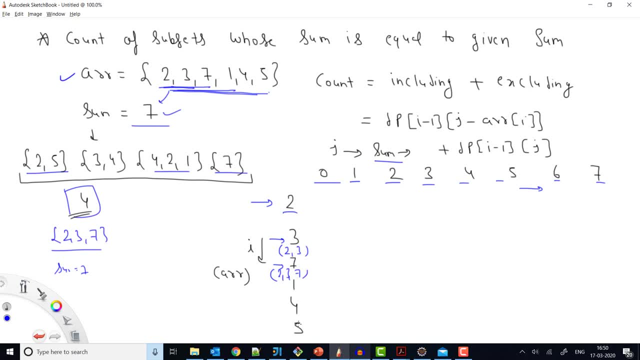 element. let's check when you have only one element. let's check when you have only one element. let's, when you have only two element, then three element, four element, five element and six element. right, so this is basically. i have explained you that how we are defining, how we are defining our dp. 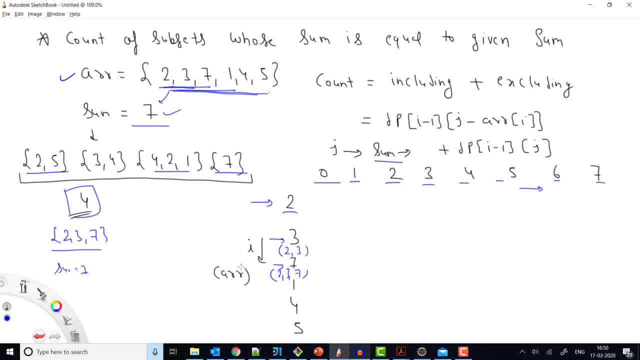 bottom of solution and when i am, when, when i am saying this row, then what it is representing, and when i am defining sum as here, then what it is representing. right now, if you see for each array element, either it will be in the answer or it will not be in the answer, right? so we can have. 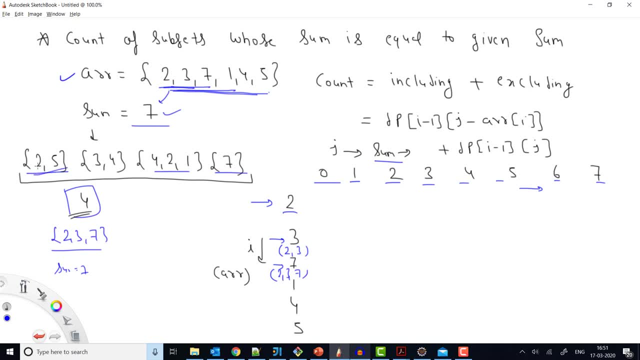 both the cases, like if you see here: here we are including only 2 and 5, but not other element, here we are including 3 and 4, not other element, here we are including 4 to 1, but excluding other element, and here we are including 7 and excluding other element. right, so it means, whenever we are, whenever 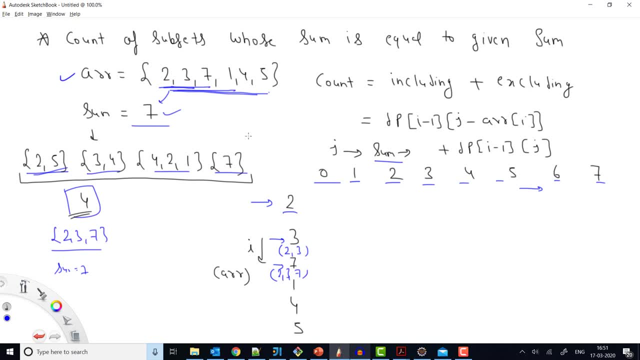 we are on a particular element, either it can be including in the subset or either it can be excluding in the subset, which is my answer right. so this is why we are saying that to calculate the count we need to take care both the cases, when i am including the current element. 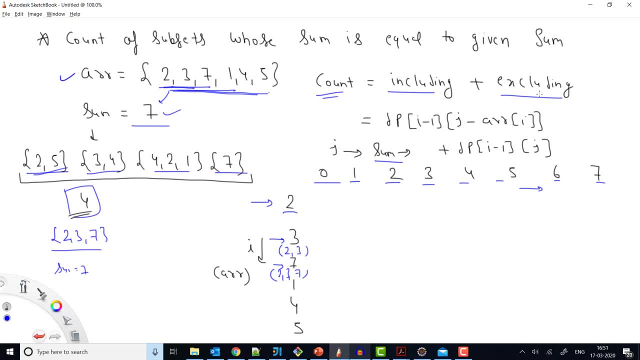 and when i am excluding the current element and whatever will be the value of the both. that will be my answer, right? so basically, i will fill. i fill the values of this matrix according to these values. so here you see, here we have including and we have excluding. now, if you see, 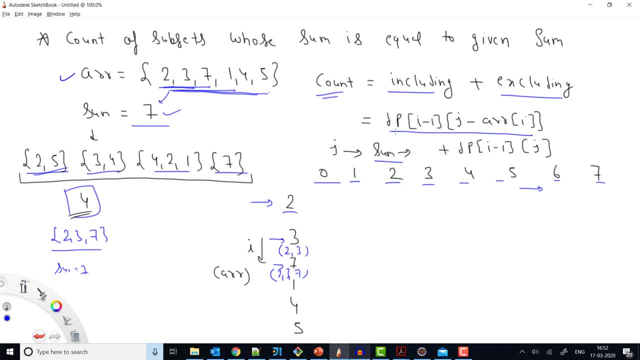 this is including. so what it means. it means basically, this dp is basically this complete dp. this is this two d array, right? so now, if you see here that if we have used one element, then it will not be repeated, right, it's just like we solved using bounded knapsack or zero one knapsack. 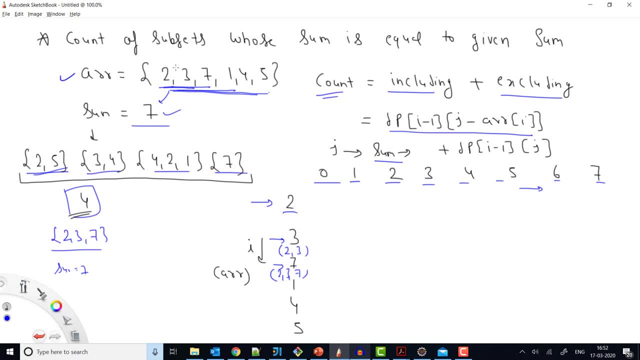 so in zero, one knapsack. what happens? that once you have chosen the one element, then you cannot choose the the same element again and again. so like, let's say, you can say here that here i have seven and here i have two, so you can say i can have one, one segment like this: two, two. 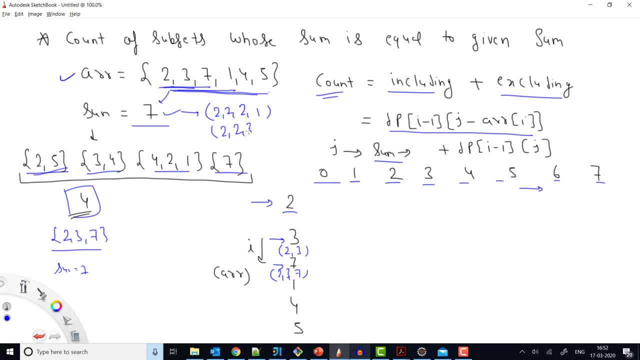 two, one. right, then you can say: i have, i can have two, two, three right now. if you see here what is happening here, i am using this two more than one time. right. here again, i am using two more than one time. so if you use, if you do something like this, then this is unbounded knapsack. unbounded knapsack means: 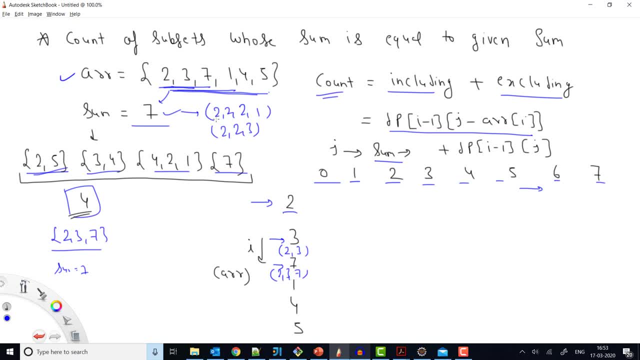 you are basically using a single element multiple times, but here when we talk about subset, so it is understood that i can use. i will use the one element only once. i will use the one element only once in my subset, like, if you see, here i use two, here with five. 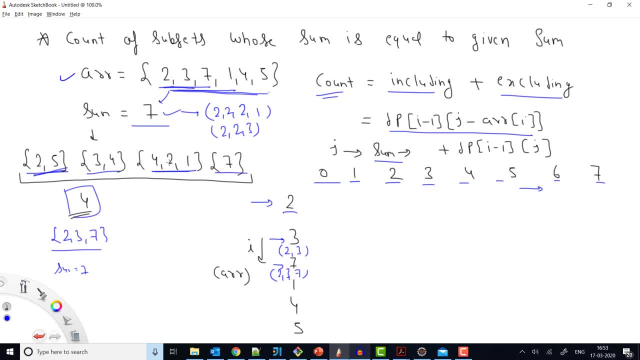 only one time now here again. now we are using two here, but it is with the different element. so this is what it says: that if i am including the current value, it means i have included the current value. so the remaining value i have to count from the previous elements. so that is why it says i minus. 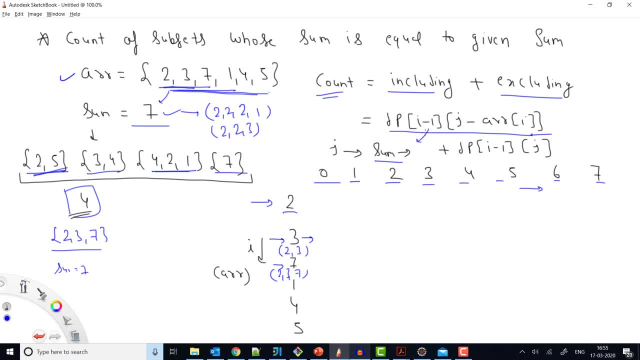 one. i minus one means i need to calc, i need to identify the remaining element from the previous, from the previous row. so that is why it says i minus one. and now why it is j minus area of i. it says: let's take one example, let's say here, if i am here, right, so if you are here, it means. 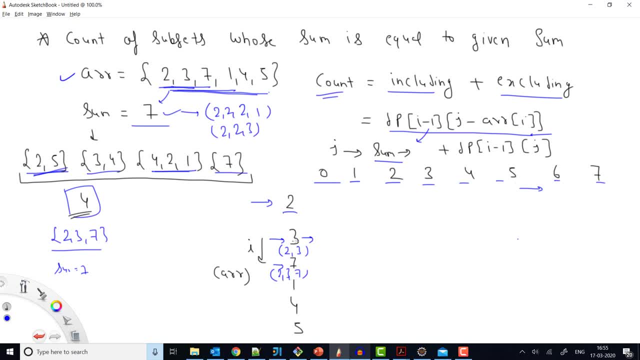 it says that if you want to get some five, then i am including this three, right? so if you are including this three, it means you have included three. so what is remaining? so remaining elements are two, because five minus three, right? so it means i will check that. what is the count of? what is the count of two? what is the count of two? and? 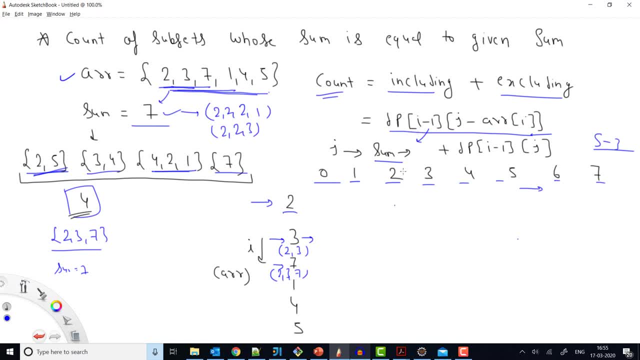 i will check it from the previous row. why previous row? because i have taken already this element so i cannot take it again. so that is why i minus one right. so this is why we have this dp i minus 1, j minus area of i when i'm including the element and when i'm excluding. 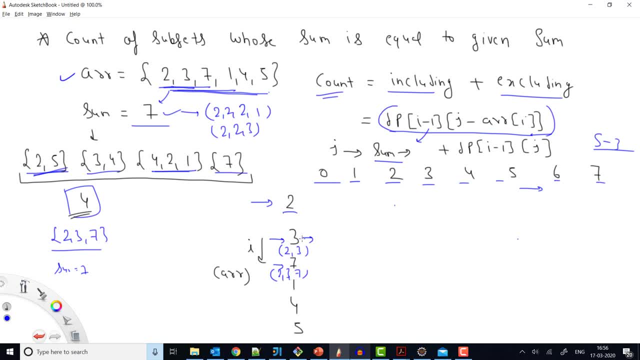 the element. excluding the element means i'm not using this element to make some. so let's say here, if I want to make 5 and if I am excluding this 3, it means I don't want to use this 3 in my subset. so it means, whatever the value of the previous row, just assign that one with the same column. 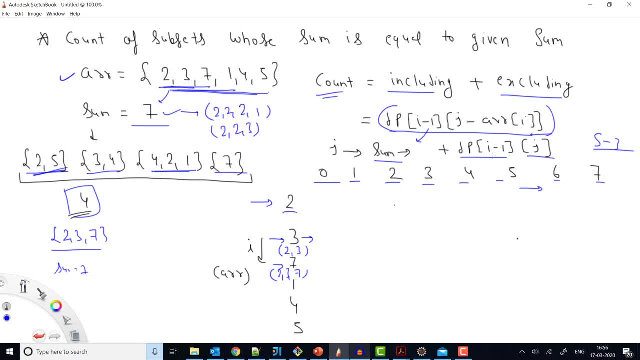 so that is what it is saying: dp: i minus 1, i minus 1, with the previous row and with the same value. same value means the same column g, right? so now, when we'll fill the value, then we'll understand it more, right, but this is what is. basic concept is now, let's fill the value 1 by 1. so now let's. 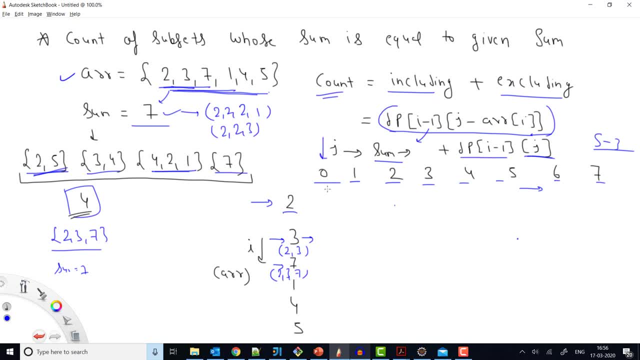 take some of the basic cases. let's take this one. it says that: how many subsets are there, how many subsets are there whose sum is 0 right now? let's say that if I have only one where, if I have only two, then how many subsets are there right? so basically, by default, what we can say. 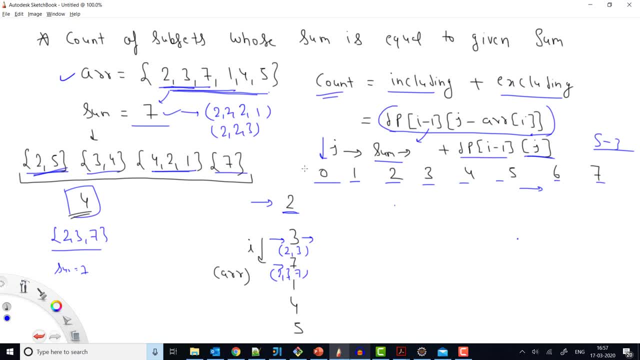 that if you want to make some 0, 0, then what you can do, that just put nothing right. it means you have one subset there that if you don't don't put anything, so that will be your subset right. so it means for all the values we 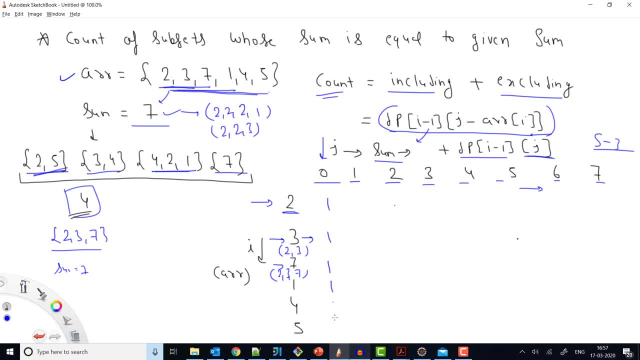 always have one subset. one subset means- which is blank subset right- that if I don't put any value, then I can make that as a subset right now. this is. this is for the 0 column, when I want to make sum as 0. now let's check this one. 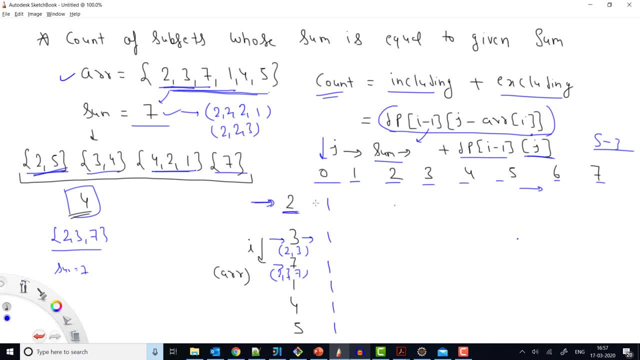 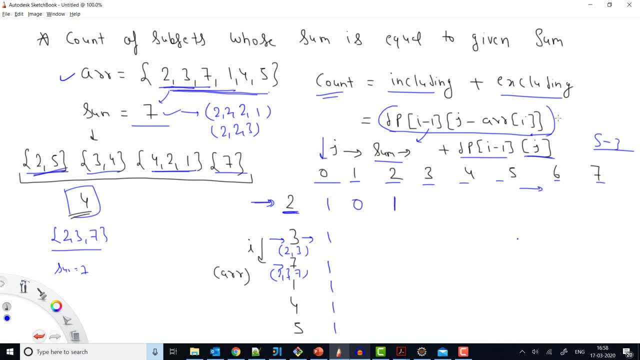 and for this value there will not be, there will not be any excluding, because i have only one value. now let's check this one. if i have only one value, if i in my set, if i have only two, can i make three? no. can i make four, no. can i make five, no, no, no. so for all the values, it will be zero, right. so for 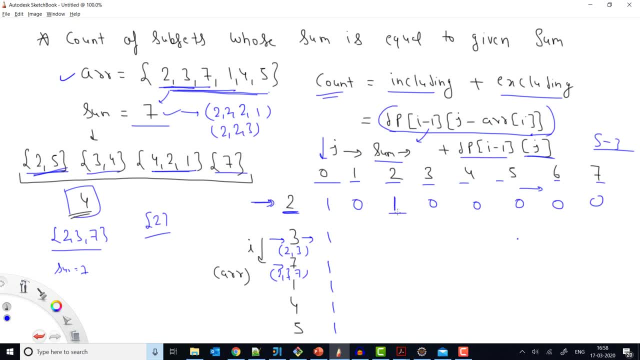 the first row, the value which will have the equal value. only that value will be one, otherwise all values will be zero. right now let's fill the other values. now let's check with this row. so in this row my value is three. right, so it means i can have two options: either i can include this or i can. 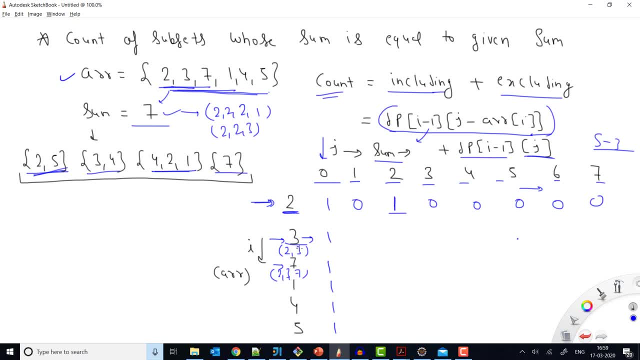 exclude this right now. i can include this value if my sum is greater than or equal to the given value, right? because if my value is less than this one, then obviously there is no point of using this, because my sum is, my sum will be less than this one. so when sum is, 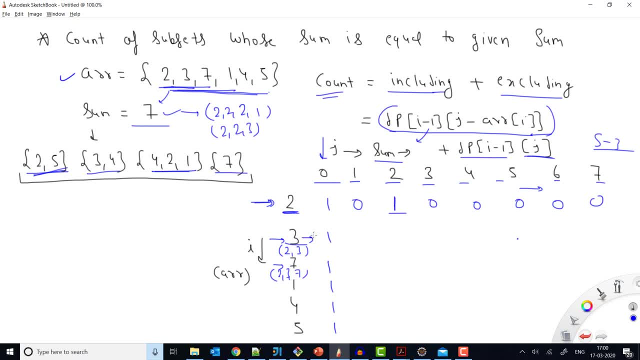 less than this one, then obviously there is no point of using this, because my sum is, my sum will be less than this one. so when sum is less than this one, then obviously there is no point of using this one. less than the this value, the current value, then in this case i can only exclude the value, not 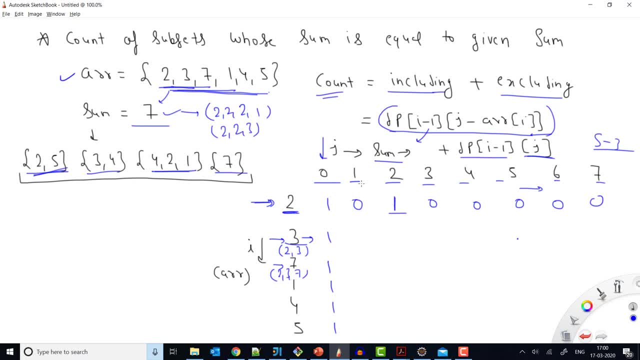 include the value. right. so now, if you see for one, so one is less than this one, it means for this i can only exclude the value. and what is the excluding value? the previous row value with the same column. so this is zero. so i will add zero here now for here also because the two is less. 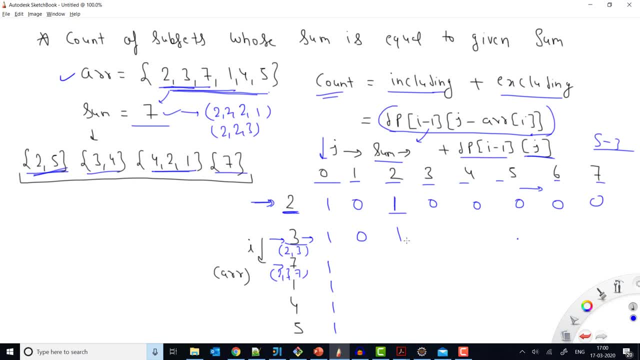 than three. so again i can add the same value, which is one. right, so it means. so why we basically, why basically, didn't include three? because i want to make sum two and my current value is three, so i cannot include this value because this is greater than this one. but now for this three. so if i want 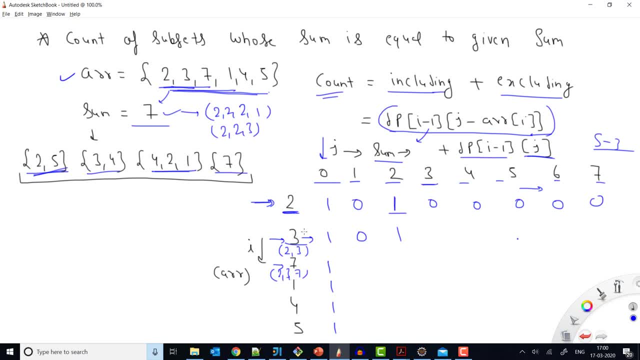 to make sum three, then i can include three, right, because my value is greater than equal to the current value. now, in this case, if you see, i'm saying that if i include the current value and my sum is three, so what is remaining? so it means remaining is zero, right? so basically i will. 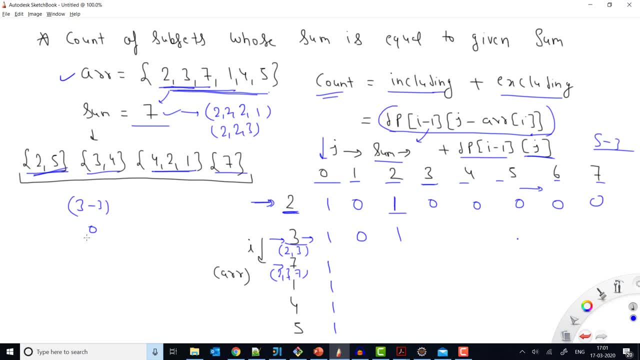 check the value of this sum and i will add the value of the current value and i will add the that. how many counts are there? if I want to make 0 from the previous row, why previous row using this one dpi minus 1, right? so previous row, there is one. it means I can make 1 and because for 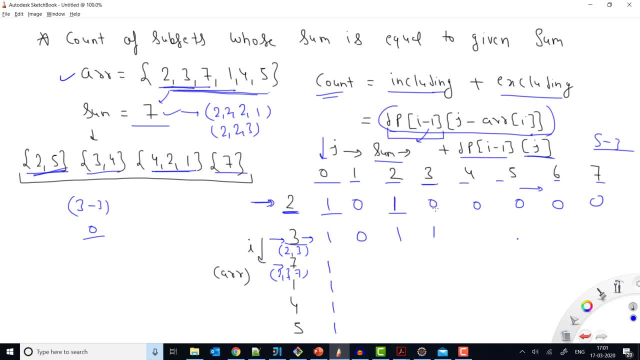 excluding it was 0, so it means 1 plus 0, 1. so it says that if I want to make some 3 and if I have these two values, 2 and 3, then how many ways are there? there is only one way. now let's check for. 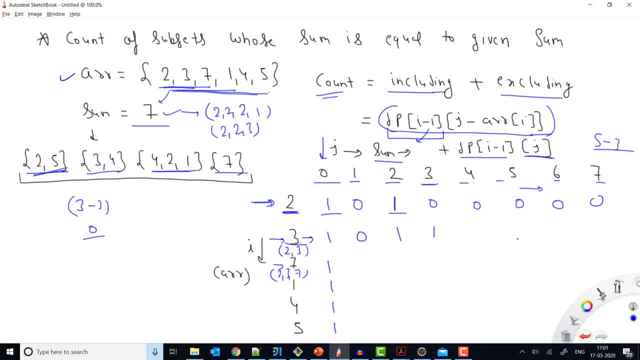 4. now 4 is greater than 3, so it means I can include the 3, so one set I have included as 3, right, so it means how many remaining values are there? 4 minus 3, 1. so it will check here in the. 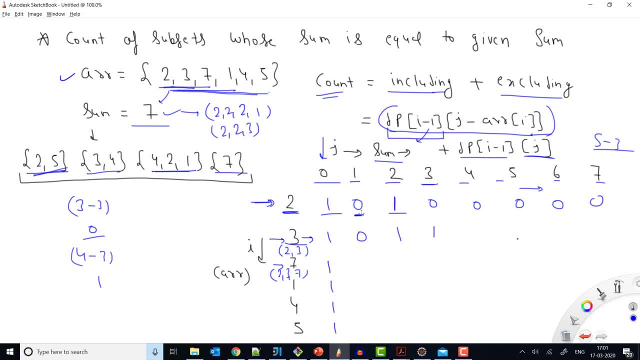 previous row. it will check how many that. how many counts are there? if I make 1, it's a 0 count, right? if it is 0 count, it means it will be 0. if I include this and for excluding there is nothing, so it will be 0, it means using 2 and 3, I cannot make. there is no substitution. 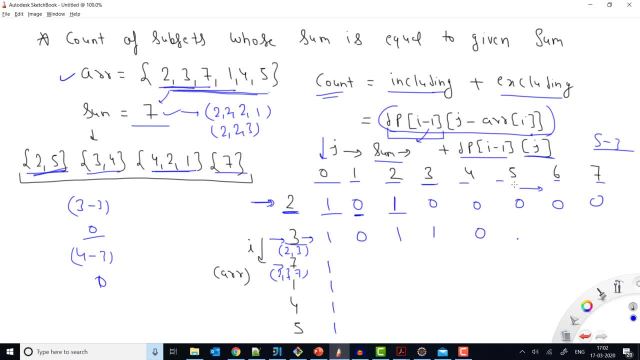 set four, which is which can make four. now let's check for 5: 4, 5 excluding is 0 and what is including? so if I include the tree, then it will be 5 minus 3, right, so it means it. check that I have taken one value is 3, now check what is the count of 2, so the 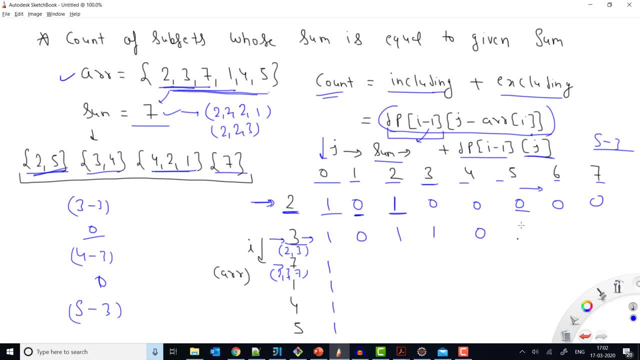 count of 2 is 1, it means 1. so it means 1 plus 0: 1. so it means out of 2 and 3 there is one count which can make 5. well, right Now let's check for 3, and here there is one count's left, so the count is 3, the count is 1. 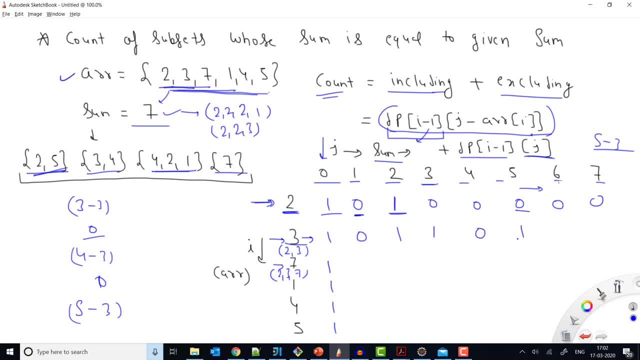 right now let's check for 2. so the count of 2 is just one count's left. so counted by 2 is not 6. so for 6, what happens for 6? we check that for excluding it is 0, so it checks 6 minus 3. 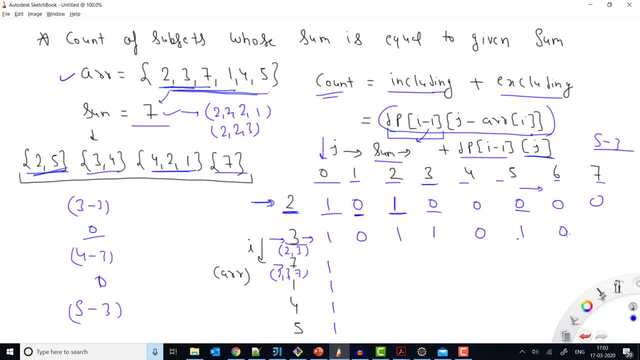 means 3, we'll check here. so this is 0, so it will be 0. now we'll check for the 7, for 7 excluding is 0, so it says 7 minus 3, 4, so it means one value. i have taken 4, just check that. how many counts are? 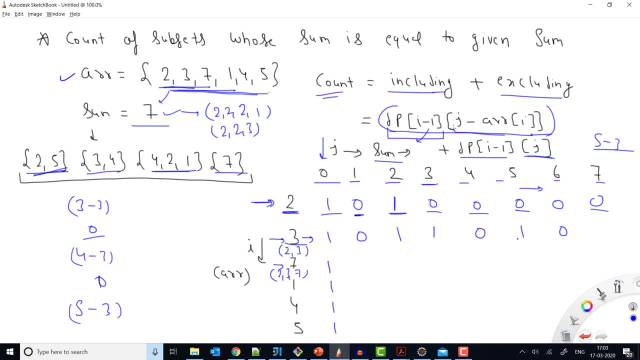 of 4 and why we are doing this using this. one j minus area of i j is j is 7. and what is area of i j is 3. so it means 7 minus 3, 4. so what is count of 4? 0 it means overall it will be 0. now my next. 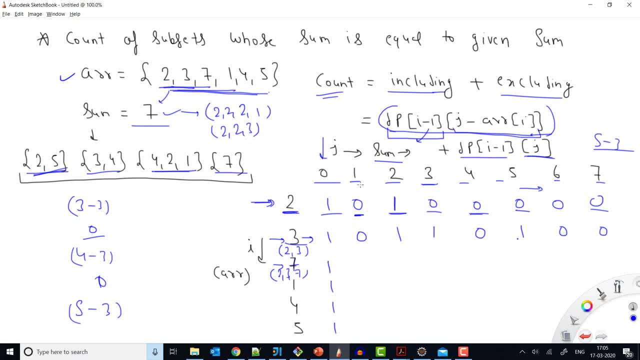 value is 7. it means: can i include 7 if i make some 1? no right, because my value, of which i am making some, is less than this one. so i cannot include this 7, i can only exclude the value. so excluding this value means previous value, so it will be 0 again for 2, also because 2 is less. 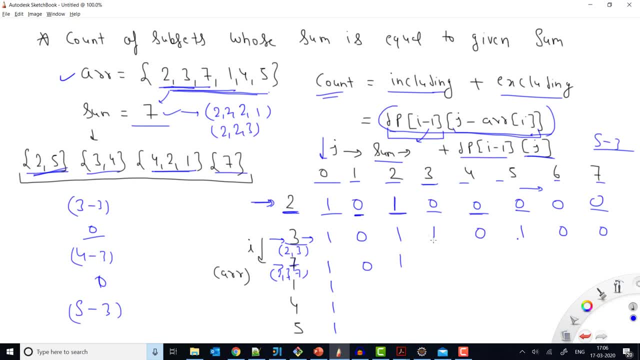 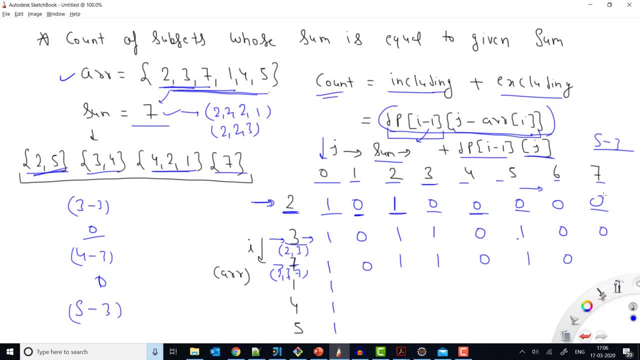 excluding this one. so it will be 1: 0, 1 0 and for 7- now it will check that- can i include 7, so 7. if i include this 7, it means 7 minus 7, 7 minus 7, which is 0. so it will check in the previous. 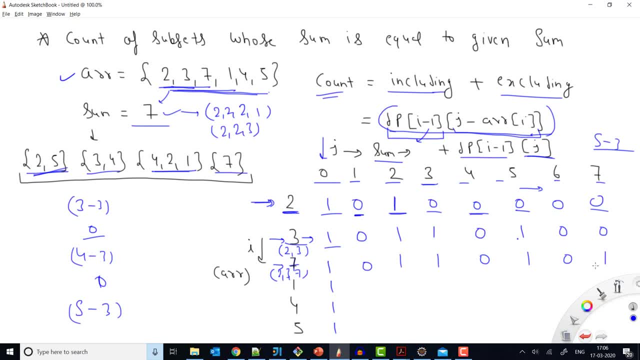 row that what is value of 0? it is 1, so it means 1. right, so it it means out of 2, 3, 7. i have only one set which can make 7, now let's check for this one. so if it is 1, 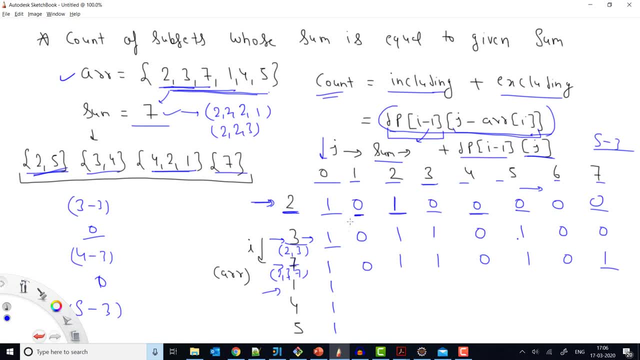 then- and here i have one- it means i can include the value. so if i include the value, it means 1 minus 1, 0, so 1 minus 1, 0, and it will check with the previous one. so previous one is 1, so it will. 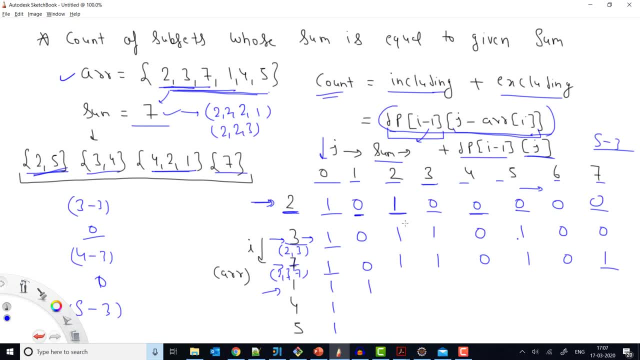 say total and for excluding it was 0, so it will be 1. now it will check for 2, so i can include this one because the value, because 2, is greater than this one. so it will say 2 minus 1, right, so 2. 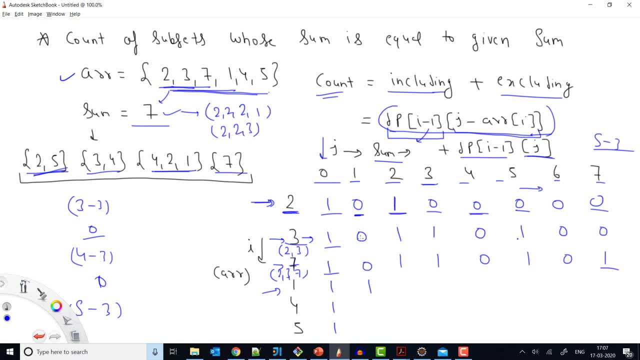 minus 1 is 1. now it will check that. can i just check with the previous one, right, because i can include this is saying 2 minus 1, which we have done, and check with the previous one. what is the count? 0, so it's a 0 plus 1, so it will be 1. now check with this: 3, so 3 minus 1, which is 2. so here, 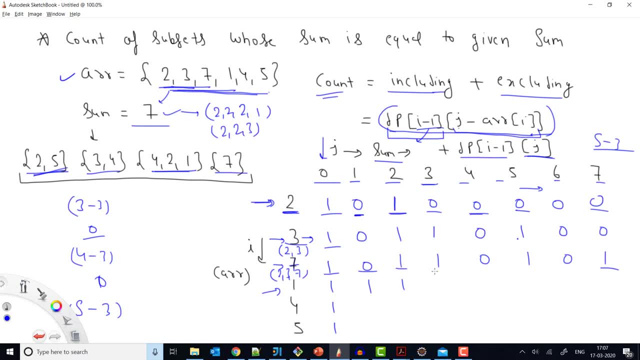 we are getting 1, so it means 1 we when we are including, and this is 1 when we are excluding, so it will be total 2. now check with this: 4. so 4 minus 1, 3. so check. is there any? how many count? 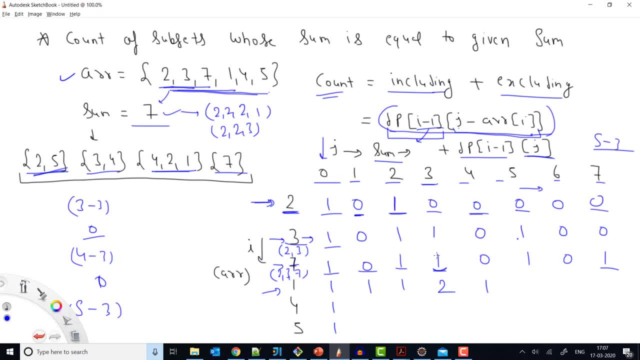 are there to 1. it means total. it will be 1, 1 plus 0- 1. so what does it mean? it means that if i want to make 4 and if i include this 1, it means 1. i have included now what is remaining element. remaining element is 3, so i will go at 3 and i will check how many counts. 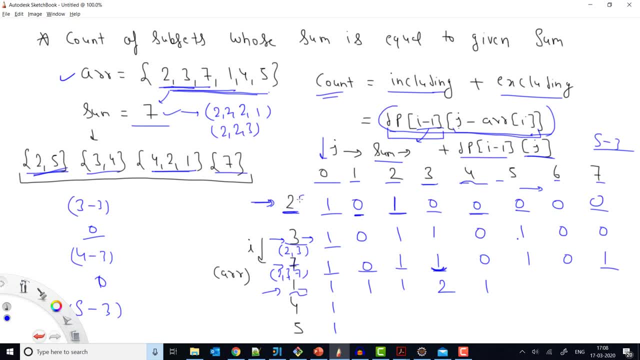 are there. if i, if i have included 3, it means with the previous values, so this is 1, so that is why i have added 1. now check with this 5. so 5 minus 1, which is 4. so check how many counts are there? 0. 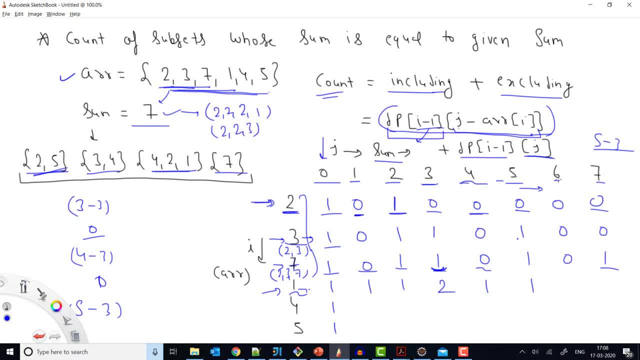 it means it will be only 1. now check with the 6: 6 minus 1, 5. so how many counts are there with the 5 in the previous row? 1. so it means 1 plus 0, 1, sorry, 1 plus. 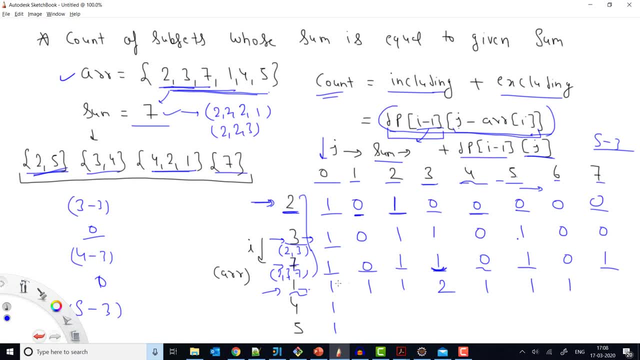 0, 1. now check with the 7. so 7 minus 1, 6. how many counts are there for the 6? 0? so it means 0 plus 1, it will be 1, right. so what we are doing whenever we are calculating for any value we are including. 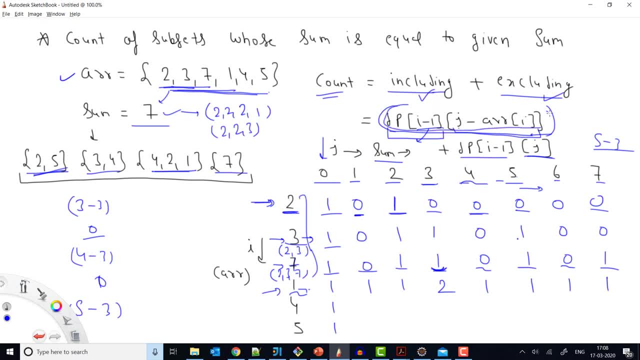 and we are excluding. so when we are including, we are following this one, when we are excluding, we are following for this one right now. check for this one: this 4 now, because this for 1, 1 is 1 is less than 4, so it means we cannot include this value, so it will. 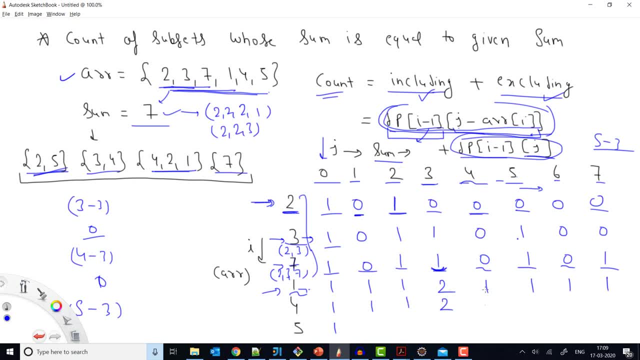 be same value which is above for 2, also for 3, also now for 4. 4 minus 4 means 4 is greater than this 4. it means i can include this. so if i include this value, so it checks what is remaining- 4 minus. 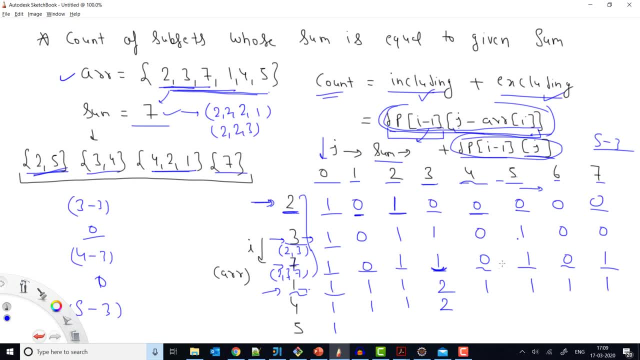 4, 0. so here we have 1, so it means 1 for the including and 1 for the excluding. so total values are 2. now you check this one for 5. so 5 minus 4. 5 minus 4 means 1. so check with the previous row how many counts are there? 1, so it means 1 and 1 for. 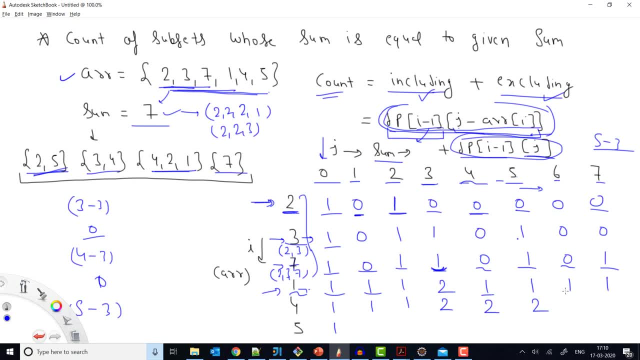 excluding, so it will be total: 2. now check for 6. so for 6, excluding is 1 and for including 6 minus 4: 2. so how many counts are there? for 2? 1, so it means 1 plus 1. 2. now check for 7: 7 minus 4. 3 for 3: we. 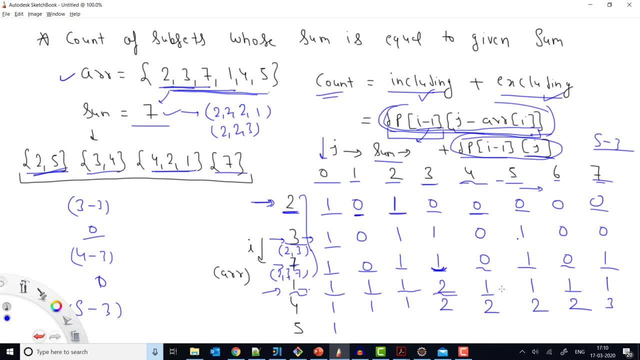 have 2 count, so 2 plus 1, 3. right now we'll check for this 5. so till here till 4, always we will be excluding because 5 is greater than this 4. so it really 1, 1, 2, 2 and now check for 5. now for: 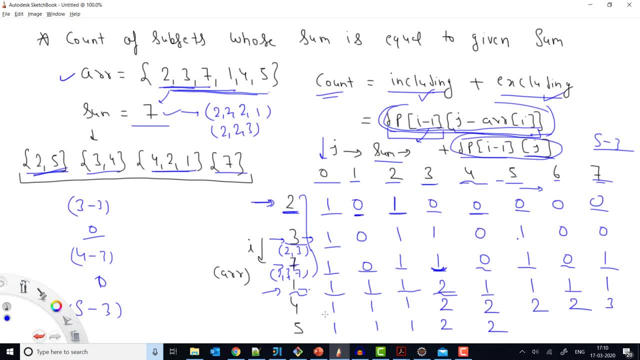 5, it will be 5 minus 5, 0. so 0 means with the 1, so 1 plus 2, 3. right now check with the 6. so for 6, excluding is 2. now it will say 6 minus 5, 1. so for 1 it is 1, so 1 plus 2, 3. now check for 7, so for 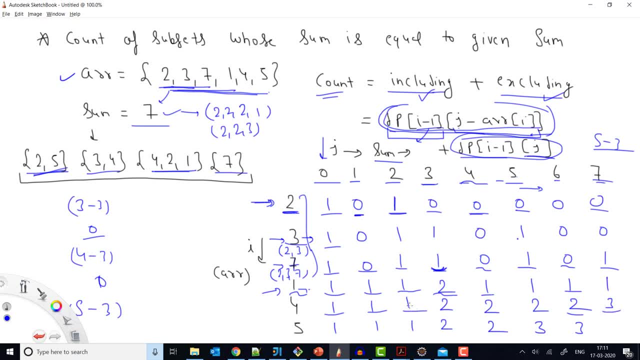 excluding, we have 3. for including 7 minus 5: 2. two, we have one, so total we have four. it means my answer will be this one, right? so this is how, basically, we fill the value and this is how, basically, at the last, we return the, this value. 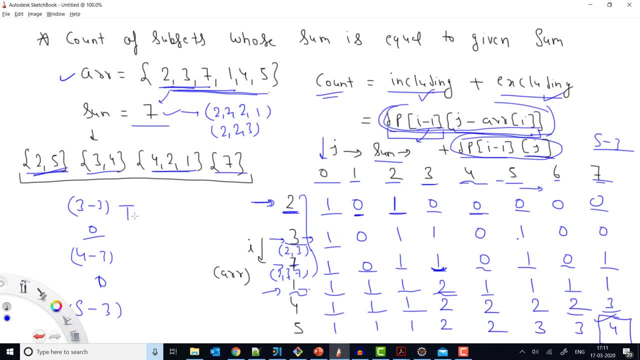 right now i should talk about the time complexity of this question. so time complexity will be: we go of number of element, where we have n and the sum which we are calculating, because till the last we are getting the maximum sum, and this will be the space complexity as well, because for this 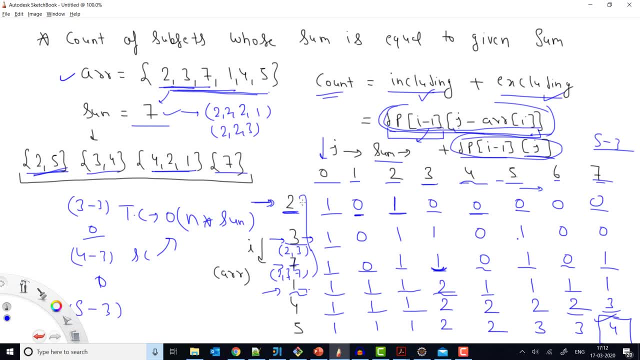 first, complexity. always, we are also taking 2d array. 2d array of the array element cross a maximum sum right. so for both time, complexity and space complexity will be and cross up. right now let me show you the code as well, so that you can get it better. 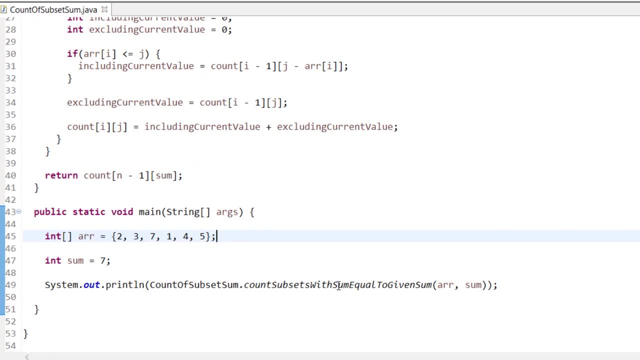 so here we have array values and here i have sum, and here is my function count subset with sum equals to given. so where i am passing here, here is my function. okay, so now i have some, and here is my function count subset with some equals to give. so where i am passing. 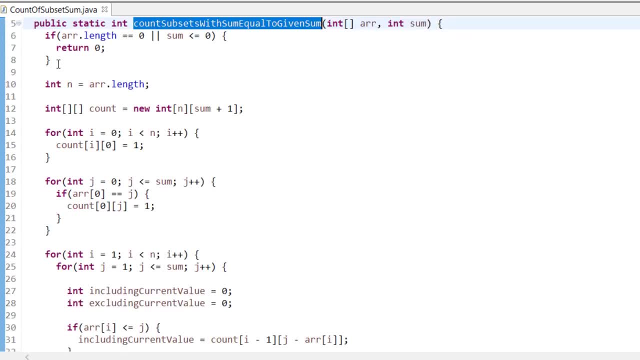 the array and sum. now these are some negative test cases, that if my array length is zero or if my sum is less than zero, then i return zero and this is how i get the array length. now i create the matrix. so my matrix is this one count where i'm passing the n. so n means the array element. 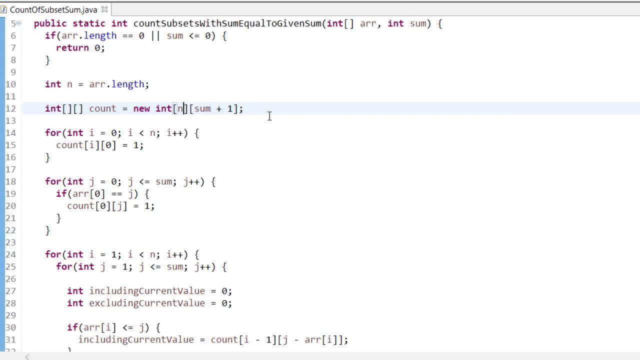 and this sum plus one. why sum plus one? because we also want to take care of zero one, the zero case, right, which is the first column. now, for the first column, our answer would be one: so this is what we fill: that for the first column, for all the rows, just fill it one now. this is for the first row. 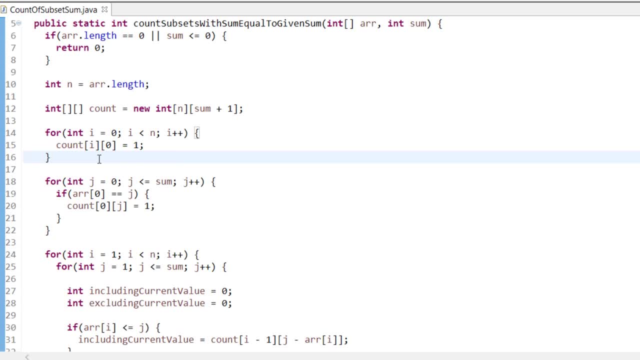 now for the first row. i will explain that the value will be one only when my value is equals to the given j, the sum value. otherwise it will be zero for all. so this is what i'm checking: that if array zero means if the first element, if my first element, is equals to the, the sum value, the. 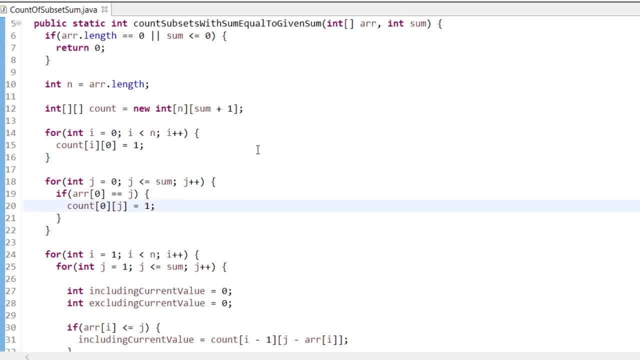 j, then only do one, else it will be zero, right? because in java what happens? that whenever we, when we fill the first column for all the rows, just fill it one. now this is for the first row. whenever we create any array, we create any array or 2D array. 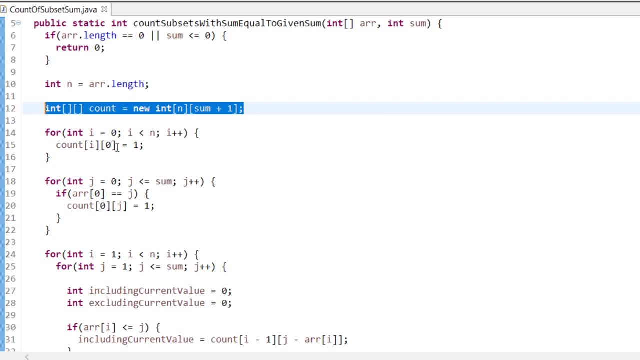 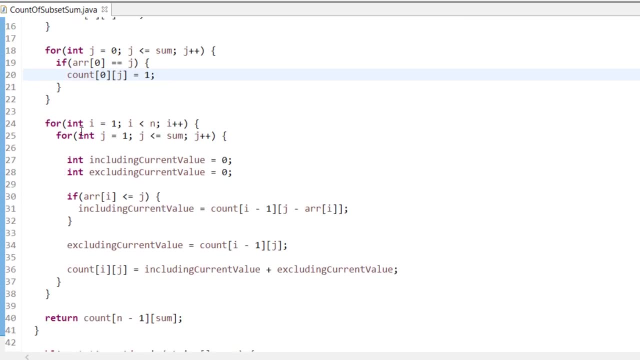 by default, all values will assign to zero for integer. So that is why for others value it will be zero by default and for this one we are making it one right Now. basically, we'll fill the values for others values Now, as we explained that we'll have two values. 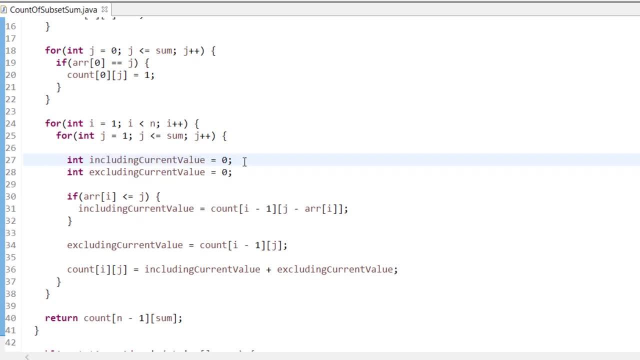 including current value and excluding current value. Now including current value: at the starting we assign both as zeros. and now for the including what, we say that if my sum is greater than the current value, the array value, then only I can include this value. 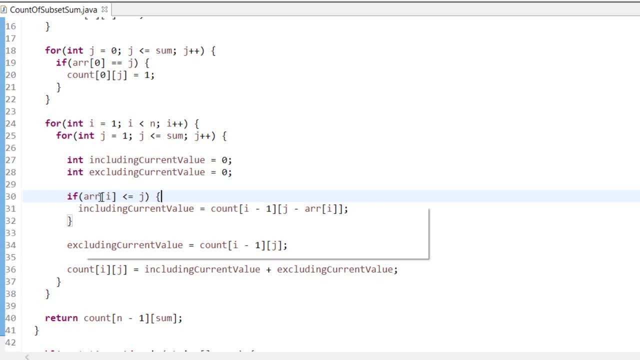 So that is why I'm assigning the condition that if j is greater than equals to the current array value, then you assign: including current value equals to count i minus one j minus array of i. For the excluding it means just for the previous value. 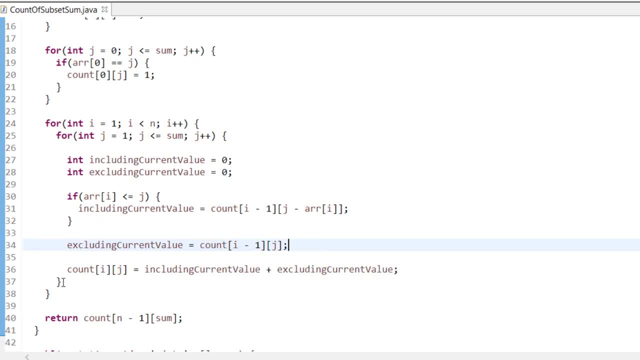 for the previous row. So that is why count i minus one j right. And at the last we assign the value, we add both the values including current value and excluding current value, And at the last, whatever is the last column, last row, value. 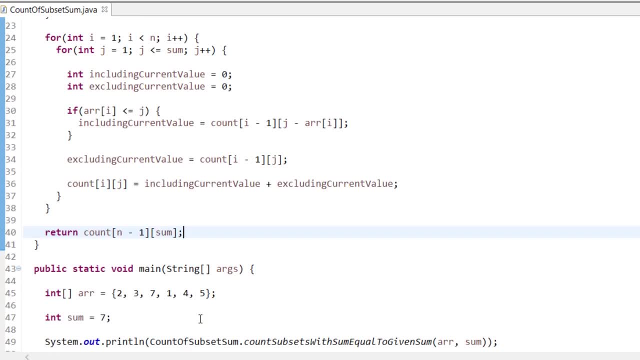 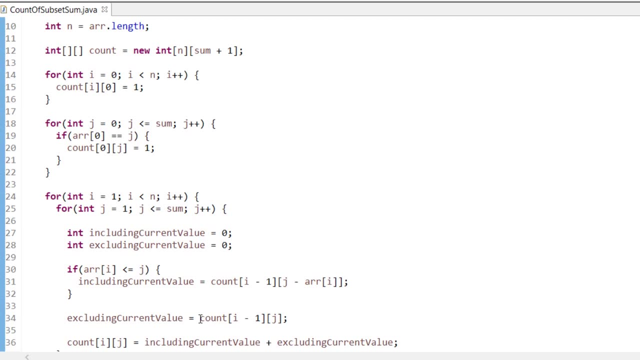 that I assign as a answer, right? So that's all, guys, about this video, and if you have any doubts, please write in the comments section and I will try to explain that, And I will also put the source code into description section, so if you want, then you can also get it from there.